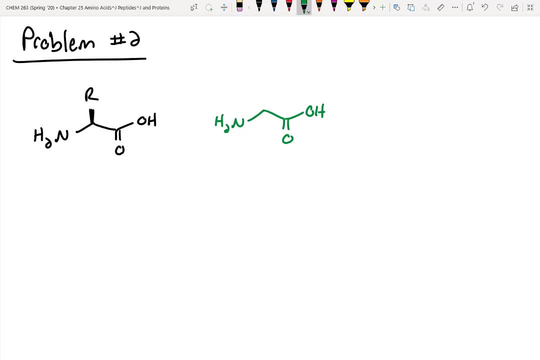 that look like this. However, our main goal was to react these two ends together. right, But if we were to react this with DCC, that peptide coupling reagent as is, we wouldn't just get one product. If it makes any sense, we have sticky ends coming off of two ends of this molecule, right? So what if? 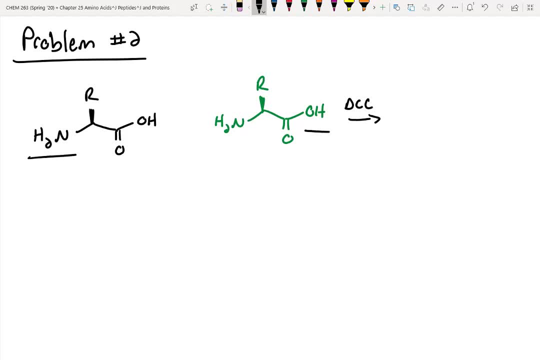 this nitrogen reacted with this carboxylic acid, Then instead of getting our correct sequence of amino acids, it would actually be inverted right. It wouldn't be the same anymore. Or we could have two of the black amino acids react together. 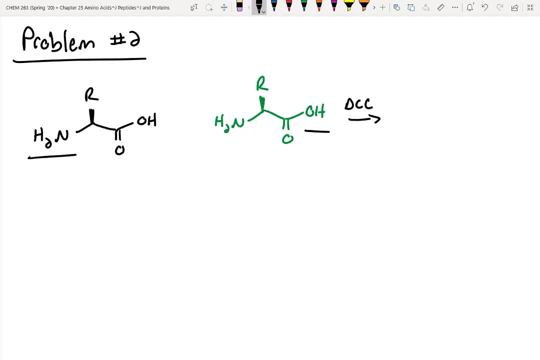 making their own unique polypeptide or dipeptide, Or we could have two green amino acids react together. So in many ways this is kind of similar to the problem we had with the crossed aldol reactions: Instead of getting one nice product, we would actually get a mix of 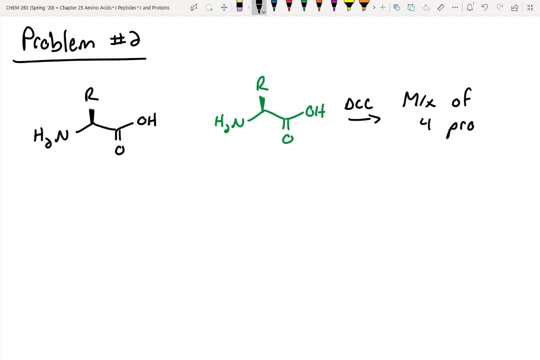 four products, Which is not ideal, right. We don't want to lose 75% of our yield due to forming three unwanted products. So, like I said, our goal is to react these two ends together. We don't want these other ends to react. 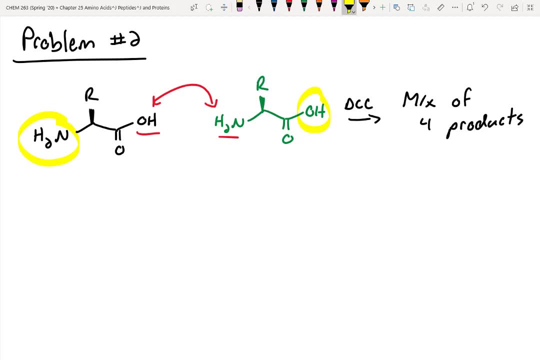 So this OH and NH2 group, we don't want to do anything. So what we need to do is we must protect these groups, And we've talked about protecting groups a little bit throughout the year. There's a ton of different protecting groups. In fact, I used to have a desk copy that went over hundreds of different. 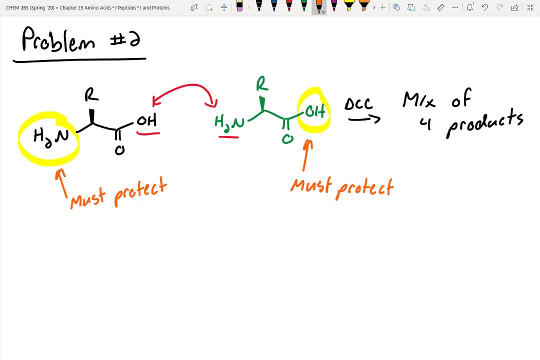 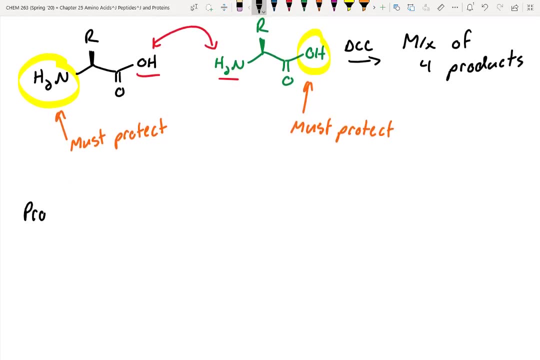 protecting groups to use for a variety of different circumstances. In this case, I'm going to show you the most common protecting groups that we use in these situations. So let's make a list. And the most common one for the smoothest amino acid. 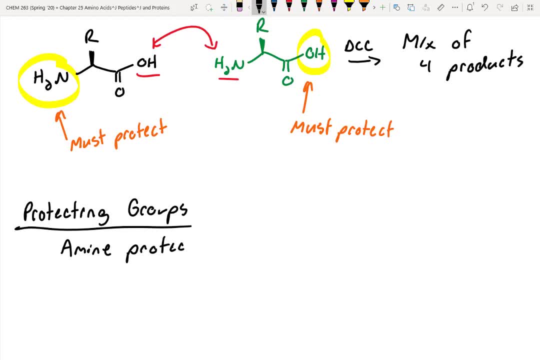 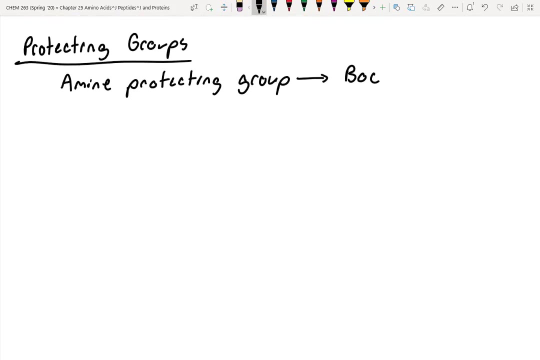 is called BOC And it's just abbreviate it as BOC, And what this stands for is TER, nee butochoide carbonyl, Sorry, tert-butyl-oxy-carbonyl. So you can kind of see the Bok in there. It's a lot easier to write out Bok than 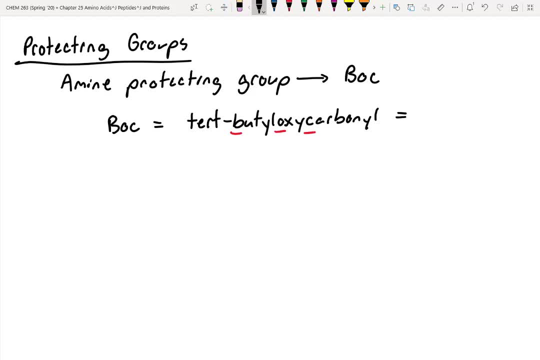 to try to explain what it is. but another way of thinking about this is it's got a tert-butyl group which looks like this: It's got an oxy group, so that's the tert-butyl-oxy, and then it's got a carbonyl group coming off of it, like 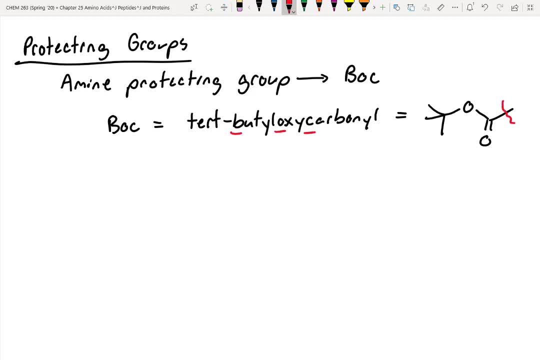 that This whole group right here is called Bok and it's normally attached to something else, So this is referred to as the Bok protecting group. As you can see, it's pretty sterically hindered, which provides some benefits too. 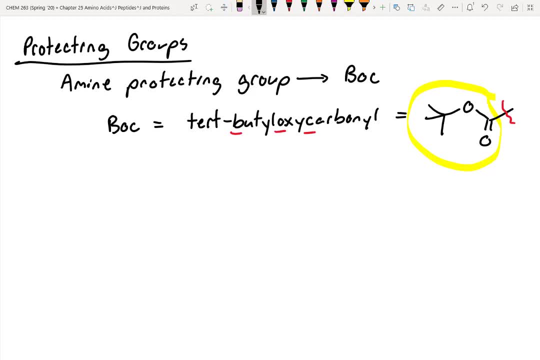 So let's take a look at what happens. if we want to install this Bok protecting group. What we do is we take our amino acid- or really any amine for that matter- and we have to react it with a specific reagent in order to get the Bok group on. 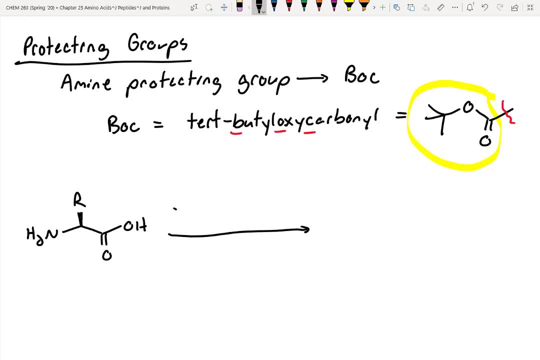 In fact, there's a couple different agents. I'll show you the most common one, though, but it's Bok anhydride, So it looks like this: So Bok anhydride, or you may see it written as Bok in. 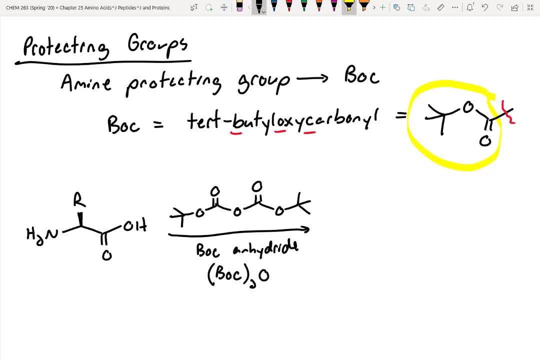 parentheses 2: O. So that oxygen right here is that center oxygen linking together these two Bok groups, right? So, as you can tell, anhydrides are really reactive. We saw this in our carboxylic acid derivative chapter and 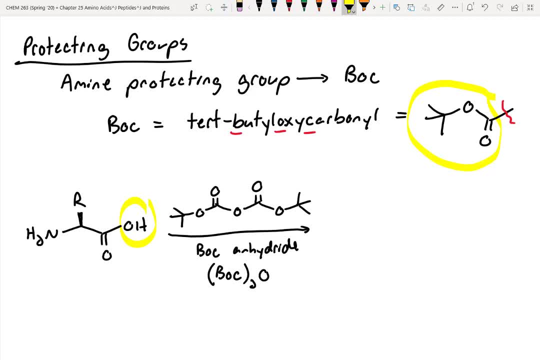 it's not going to react with this carboxylic acid group simply because this nitrogen lone pair isn't delocalized and nitrogen lone pairs are better nucleophiles, So it's going to selectively protect that nitrogen group. So let's take a look at what happens. Well, we're going to get the Bok group. 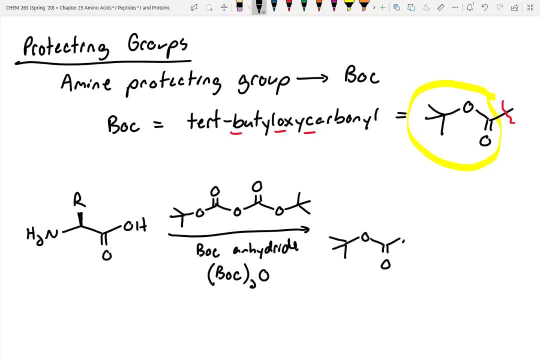 installed and we're going to protect that nitrogen. I'm going to take a look at what happens here. I'm going to turn this on and let it indicate that it's going to react with this Bok group. This is the new bond that 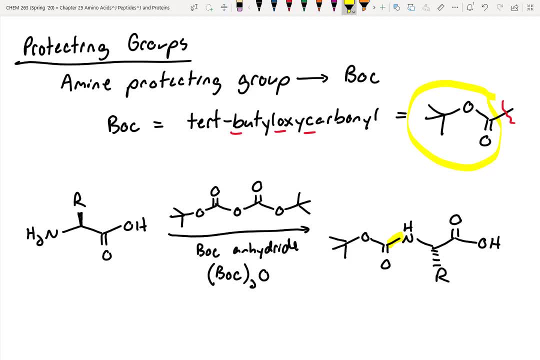 is formed between that nitrogen and our Bok group, and then this whole thing can be abbreviated just as B-O-C, if you'd like to write it that way. You'll see that shown a lot in your biochemistry courses. Alright, so we have that. 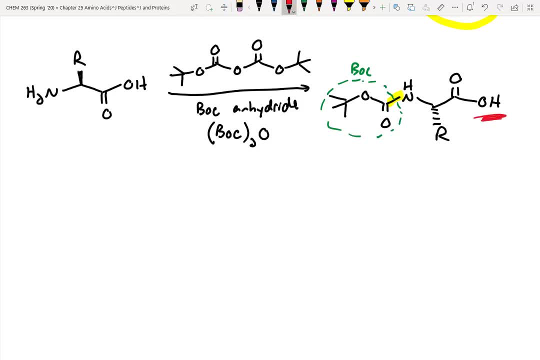 protecting group on. Now we can react this remaining carboxylic acid end with our other amino acid without worrying about the nitrogen end over here doing any sort of unwanted chemistry. all right, and then, when you're all done, what we need to do is we need 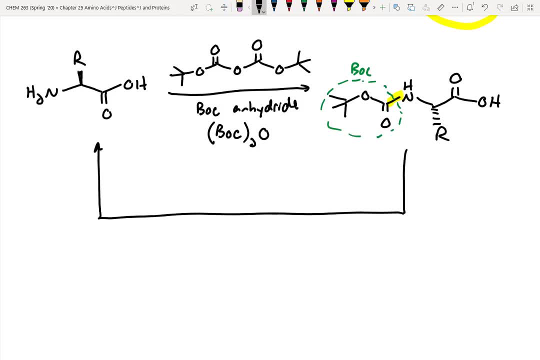 to remove this protecting group and go back to our original amine form. right, and in order to do this, we use a special acid. it's called trifluoroacetic acid. it's kind of like acetic acid on steroids. these three fluorines have a huge amount of inductive pole, which makes this far more acidic. 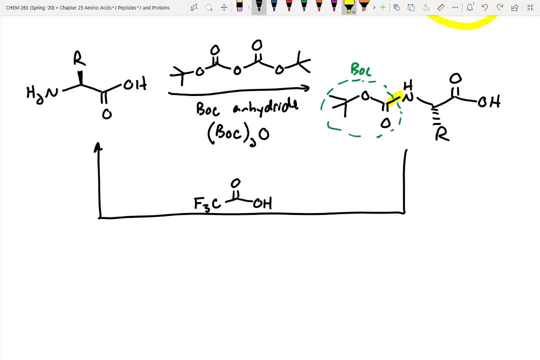 than regular acetic acid, so this works really well. like i said, it's called trifluoroacetic acid and some chemists will just simply abbreviate this as tfa. it's a lot easier to write tfa than to write out trifluoroacetic acid, so this allows us to install a protecting group and then remove. 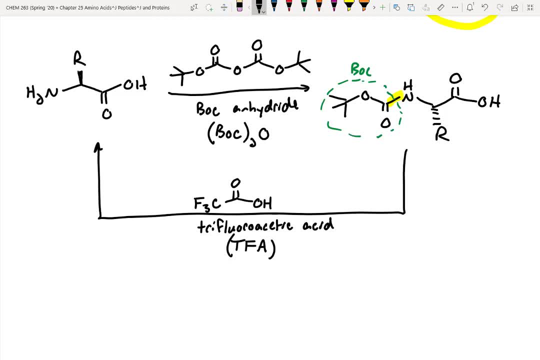 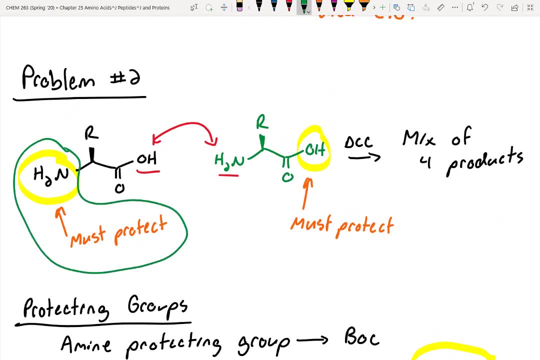 it at our leisure by using tfa, all right. so then the question is: well, we've addressed protecting this amine and amino acid number one, but how do we protect this group over here, the carboxylic acid group and amino acid number two? we also don't want that to react either. 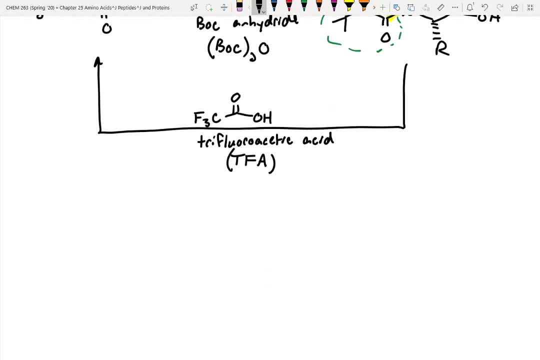 so let's take a look at that next. so this would be our carboxylic acid protecting group, and there are a variety of different carboxylic acid protecting groups, but i'm going to show you the most basic one. so let's go ahead and show our mean or sorry, our amino acid and amino acid. 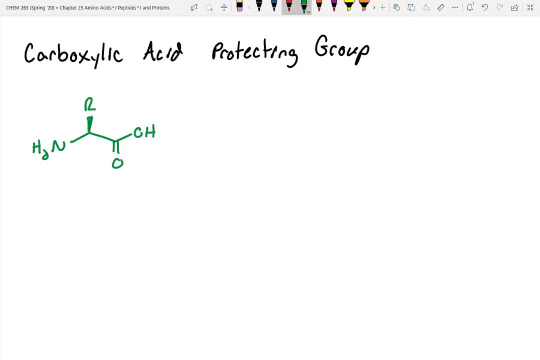 number two, right, and our goal here was to protect this carboxylic acid group. this one's actually more straightforward, in my opinion. In order to do this, what we need to do is a Fischer esterification using benzyl alcohol. So this is benzyl alcohol. 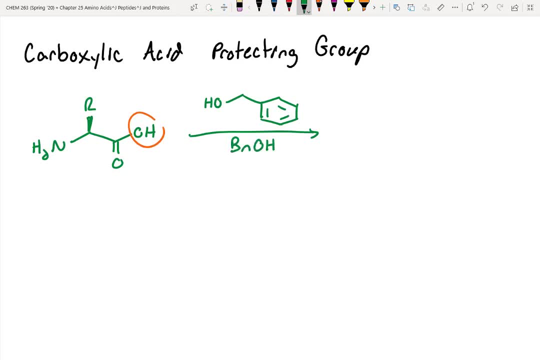 Oftentimes it's just abbreviated B-N-O-H And, if you remember, benzyl groups are kind of unique. Benzyl groups always have the CH2 spacer, So this is why we call it benzyl alcohol and not phenol, right? 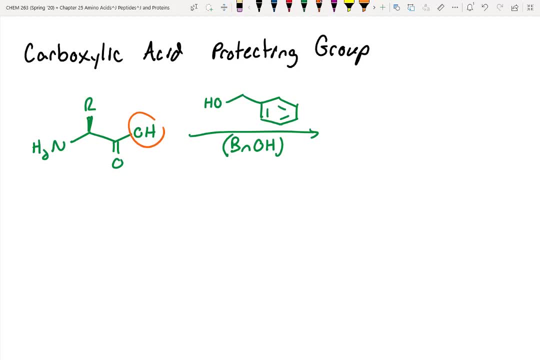 Phenol would have the OH directly attached to the ring. So in order to do this Fischer esterification, we also need catalytic acid. So in this process, what we're going to do is we're going to make a new ester group. 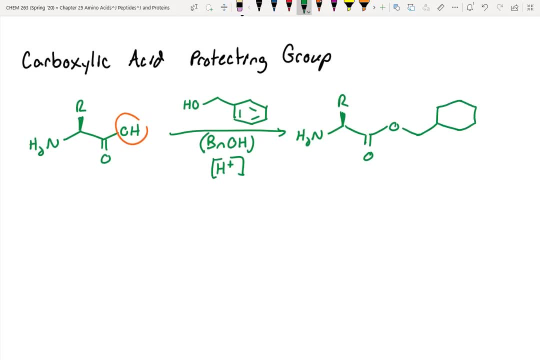 Let me zoom out a little bit. And we've got this new ester group over here. So if we want to make a new ester group, we want to abbreviate this. Oftentimes this entire group is called O-B-N. 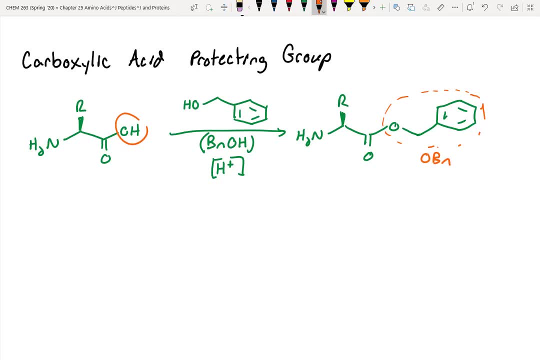 This won't do any acid-base chemistry anymore, right, Because it doesn't have any carboxylic acid, acidic proton And it's not going to do any of the unwanted chemistry with our peptide coupling reagent, So it's a good blocking group. 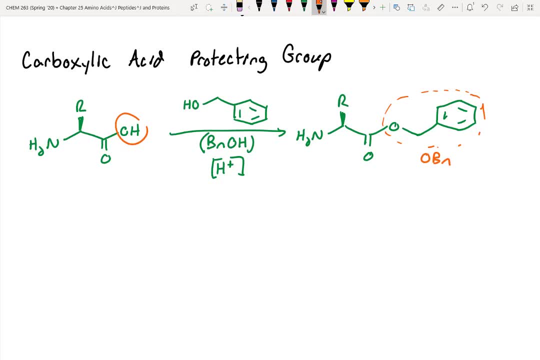 that we can install temporarily to prevent any sort of unwanted chemistry from occurring, And then, just like before, we want to be able to remove it at the end. So we can go ahead and remove it using a variety of different techniques. One is to use hydrogen and palladium on carbon. 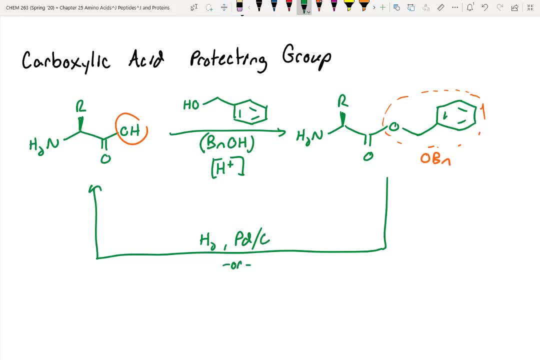 at relatively low pressures. Or, if you don't want to do that, you can treat this with hydrobromic acid and acetic acid, Or if you don't want to do that, you can use sodium hydroxide and H2O. 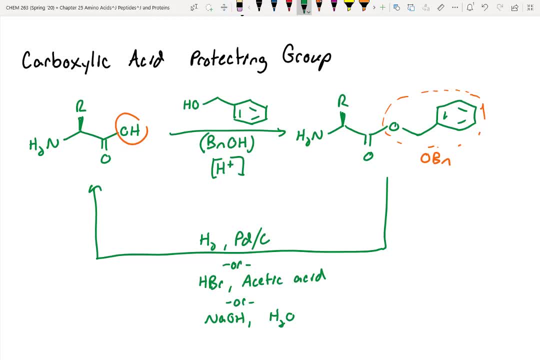 Oftentimes sodium hydroxide and H2O. you can use sodium hydroxide and H2O, But the method you use depends on whether or not you have any sort of sensitive functional groups that are sensitive to acids or bases, So you might want to select the deprotection scheme. 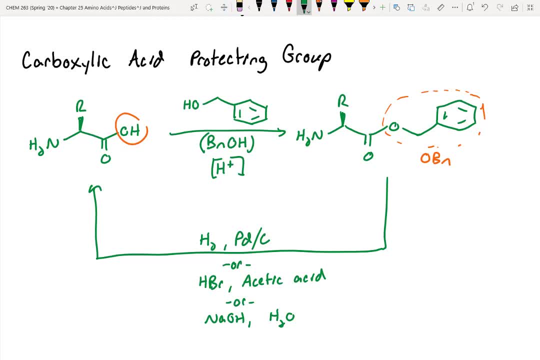 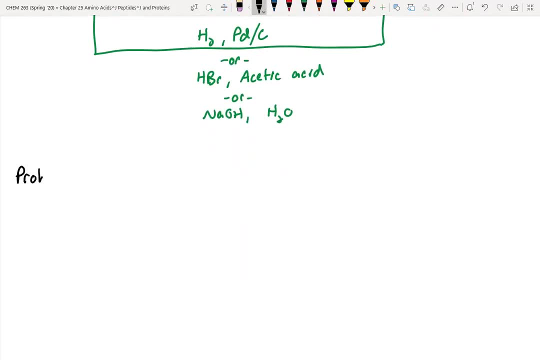 that is suitable for your amino acid side chains, All right. Problem number three is just more of a generic business problem, All right. So problem number three I'm going to break down into three parts. One is: the greenness of these reactions is terrible. 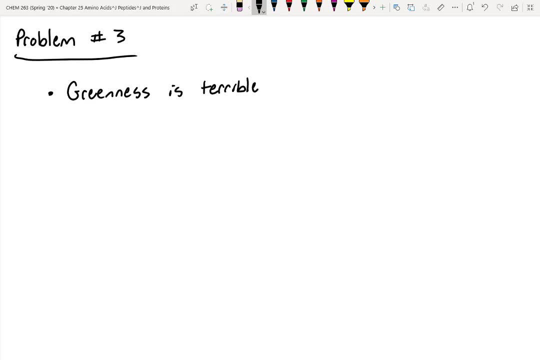 All right. If we have to install a protecting group on each of our amino acids and then use a peptide coupling reagent that has low atom economy and then deprotect our amino acids using separate chemistry, we're turning essentially what biology does in one steps. 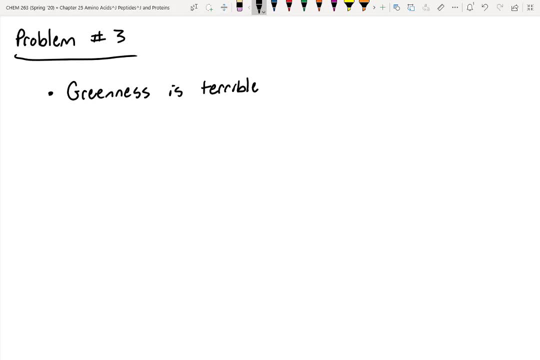 into a multi-step sequence and we're wasting a ton of atoms right. So the greenness of these reactions is really bad. The offshoot of that is the cost is really high If we try to do this on a bench top right. 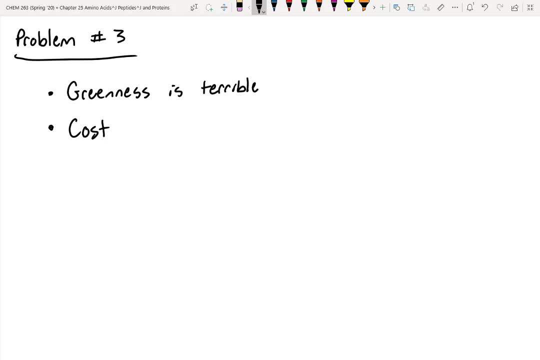 We're not only using a lot of reagents, but we're taking up a ton of time, and the time of chemists obviously costs money, right? So time is another one that is closely linked to costs. All right. And then the last one is: even if you're a really good chemist, 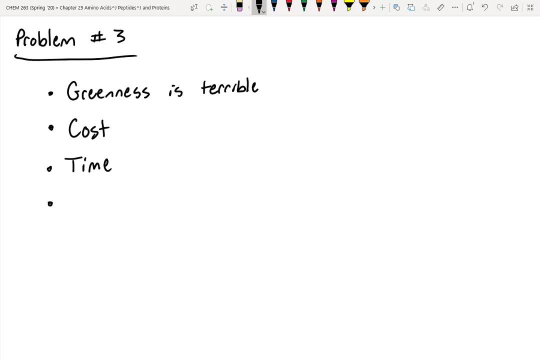 if you're stretching one reaction into multiple reactions, you're going to take a hit. You're going to take a hit and yield right. So the yield for these reactions tends to be pretty low when we do this. So I wanted to give you a specific example.